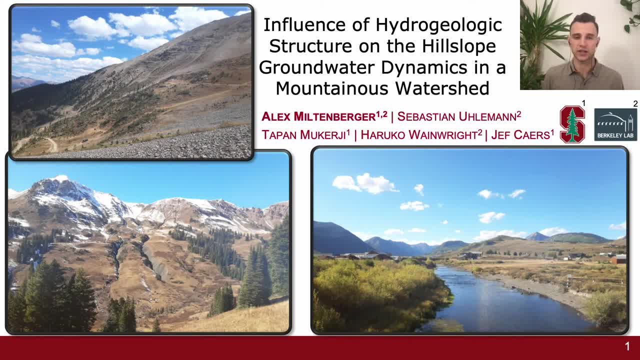 Hi everyone. my name is Alex Miltenberger and I'm happy to be sharing some of the work that I've been doing over the past six months or so with Stanford University and Lawrence Berkeley National Lab. So for this project, we've been really interested in the hydrogeologic structure. 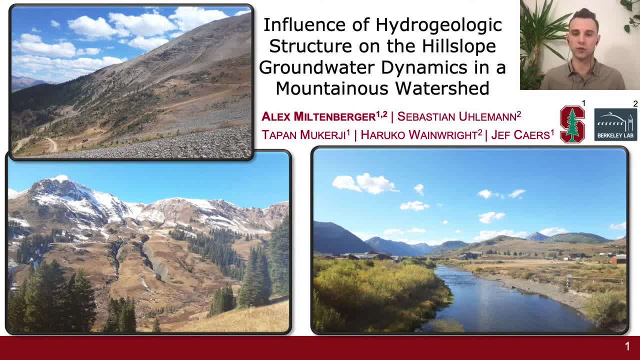 of the upper part of the Colorado River Basin, So this is where all the water of the Colorado River comes from. The Colorado River obviously feeds a huge amount of the western US with water and all of the water in this river comes from the mountains of Colorado, Utah and the surrounding. 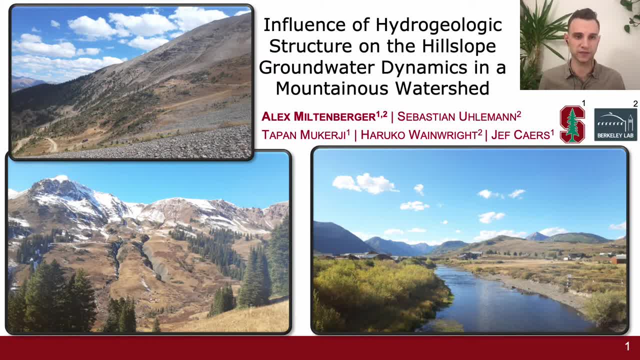 states. So I wanted to share a few pictures from a recent field campaign that we did to Colorado where we were studying the hydrogeologic structure of one of these catchments. So this picture on the top left is pretty representative of all the highest parts of 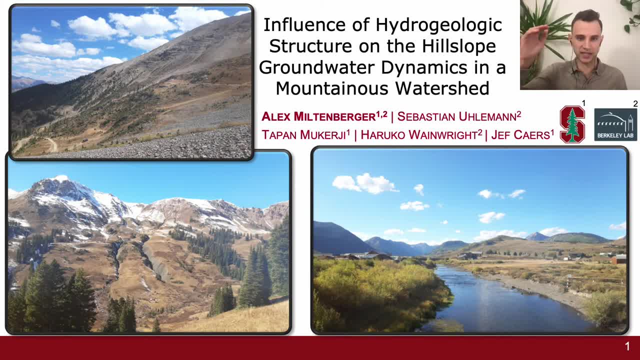 these catchments in this area. So we're up near the peaks of these mountains and we're in these glacially carved valleys that are now filled with big piles of angular, coarse, talus piles and other kinds of sediments, and then, if you follow this valley down far enough, eventually you'll hit a. 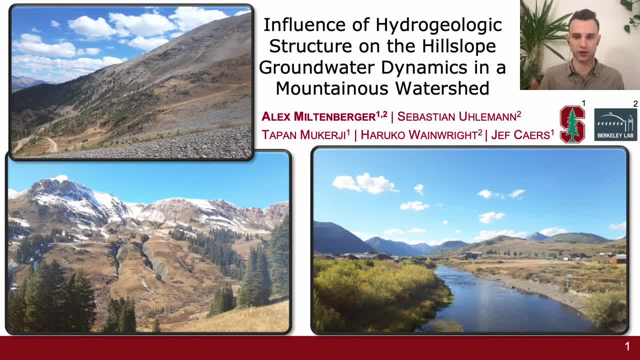 headwater spring, so this is where the water is first coming out of the ground and if you follow that spring down, you'll see more and more seeps coming out of the ground and the stream itself is getting bigger and bigger as you're getting contributions from the surrounding hill slopes. 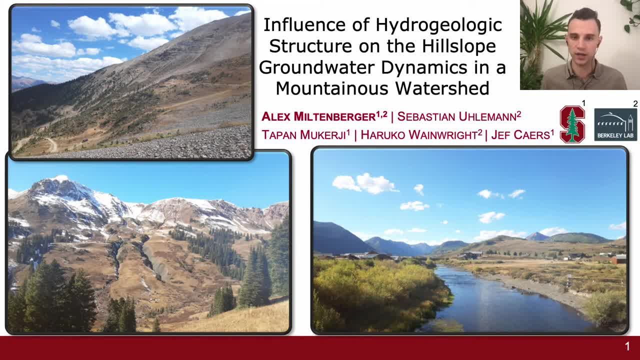 such as the one shown on the bottom left here, and so by the time you get into the main valleys, you've accumulated quite a bit of water from all of these catchments coalescing into a single river, and so that's what this figure on the bottom right is showing, and then this water will exit out to. 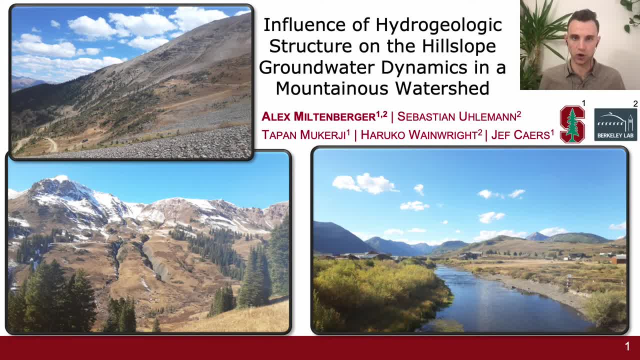 the gunnison river and then eventually to the colorado river. so all of the water, especially in the dry season, is coming from. snow melt in these, in these catchments, here in these mountains, and it's remarkable that even in the dry season, after the snow has melted, that we have this much water. 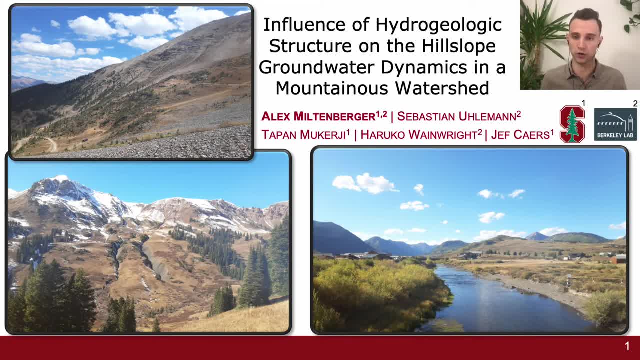 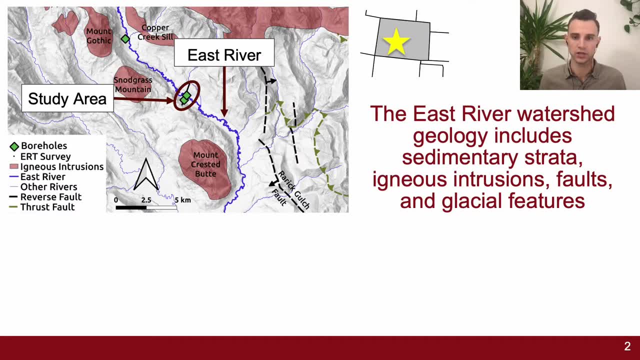 that's all being fed from groundwater. so what we're really interested in is the geological structure of this area and how that affects the groundwater flow. so here's a little bit of background on the geology of this area. so we're in the east river watershed, which is a big doe funded. 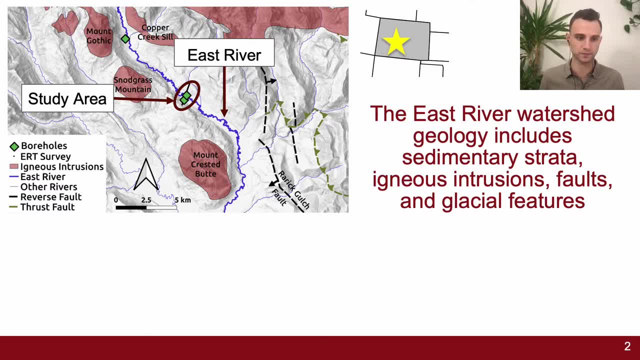 site. there's been a lot of work done here. that's shown in this star and that you can see on this picture goes through this area that's surrounded by igneous intrusions in red, and there's also a lot of faults shown as these lines with the arrows. and if you take this cross section from b to b, prime, 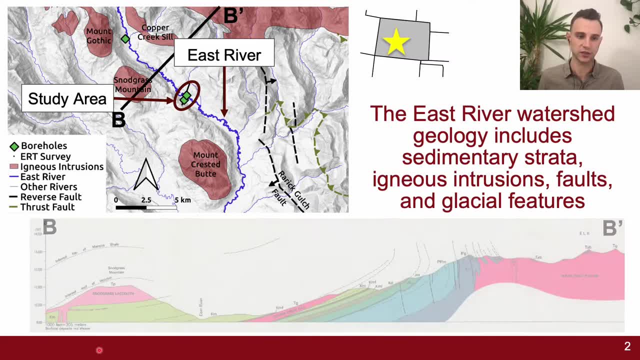 which is near our study area, which is circled here. you can see the kind of structure we're working with. so we have igneous intrusions and then we have a thick package of manco shale and green, and then we have all of these dipping layers that are dipping down towards the southwest and up at the 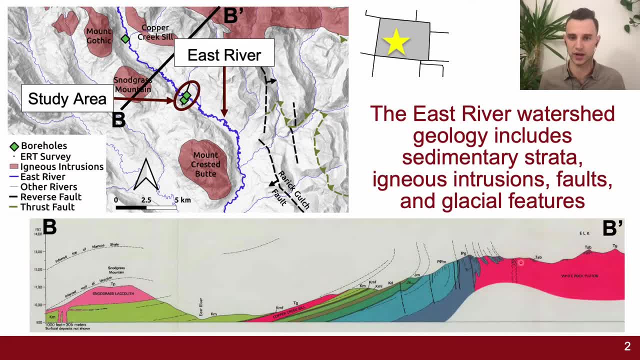 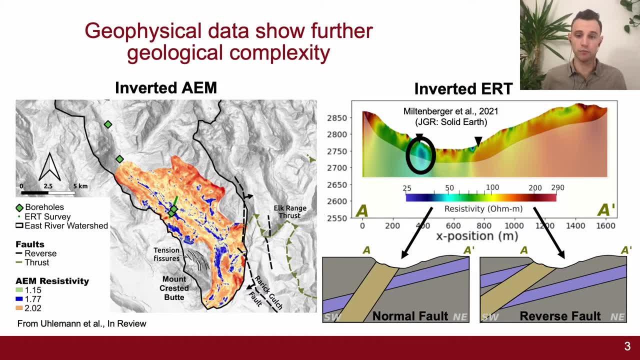 top we also have this big thrust fault called the elk range thrust. that also is associated with a big intrusive body and there's actually more complexity than even what's shown in this map, because the the some of the geological structure is concealed below the surface and it can only be 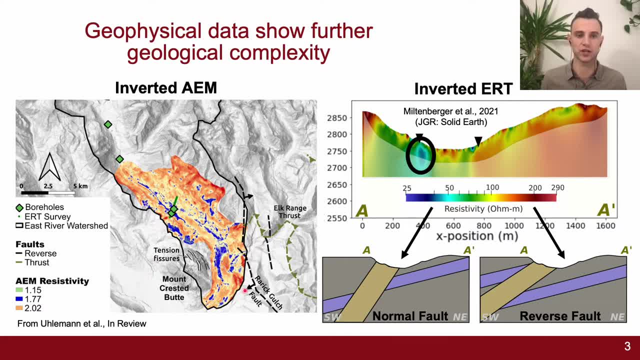 seen through geophysical data. so what i'm showing here on the left is an inverted airborne em cross section, and you can see that there's this electrically resistive or electrically conductive anomaly that runs right along the edge of the geological structure and that's the geological 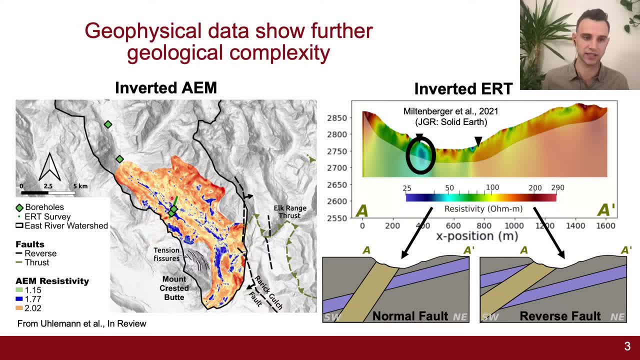 structure along the axis of the valley and if you take a electrical resistivity tomography cross section across that anomaly you see it shows up and it penetrates pretty deep into the subsurface. so we did a lot of work last year studying this anomaly and we were able to determine that it's 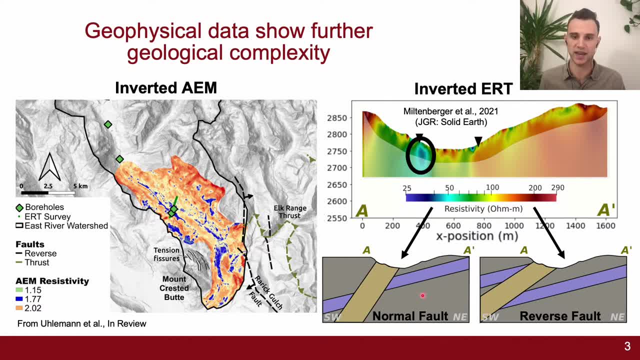 most likely either a normal fault or a reverse fault, just based on the shape of the anomaly and how consistent it is with these subsurface models. and then this work was published in jgr solid earth. but what it's left us with is the question of what other kinds of subsurface features are there? 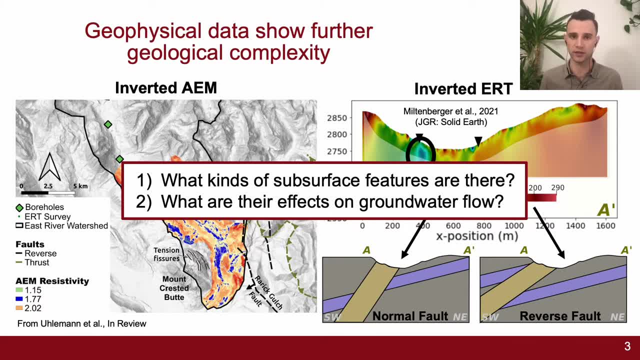 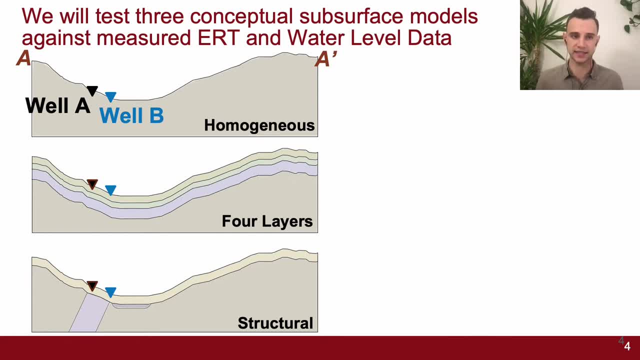 and how do these subsurface features get put into a groundwater model and then how do they affect the groundwater model? so the way that we're going to test these models or these- this this question- is we're going to propose three different subsurface conceptual models and those are shown here on the left. so 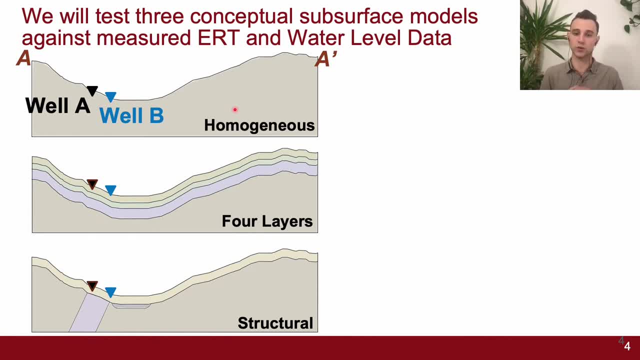 our first and simplest is a homogeneous subsurface. so we know this is wrong, but a good baseline. so we're going to say everything's the same in this homogeneous model. next we're going to use a layered subsurface model, which is a pretty common representation of the subsurface. 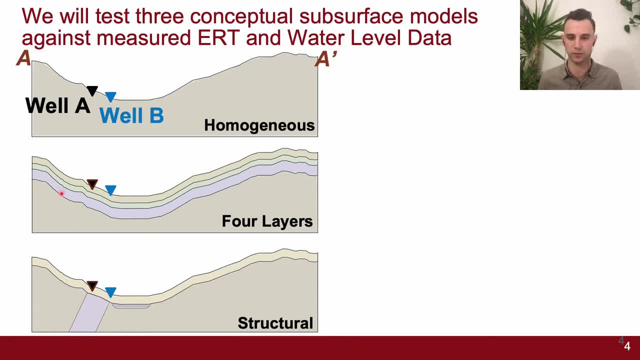 when we don't have great geological information to put into our model, we'll just assume this layered structure and then, finally, we'll use a structural model which is in the bottom here- and we call this structural because it includes this fault zone as well as the floodplain, and then a 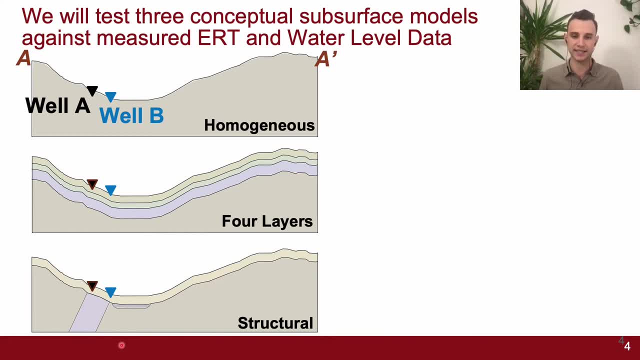 soil layer, so different structures. and then we're going to test these data, or test these models using data from electrical resistivity tomography, which i showed on the last slide. but these are the resistance measurements projected into a pseudo space, depending on the electrode configuration. and then we also have 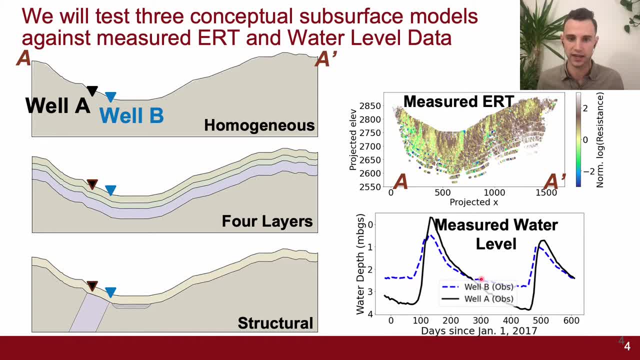 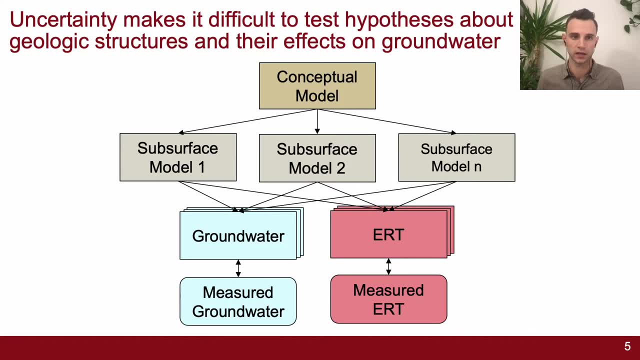 water level data at well a and well b respectively, and you can see that's over two years, as you can see in this plot on the bottom. so the challenge with evaluating these kinds of conceptual models is that we have uncertainty the whole way down. so we've already outlined that we have uncertainty. 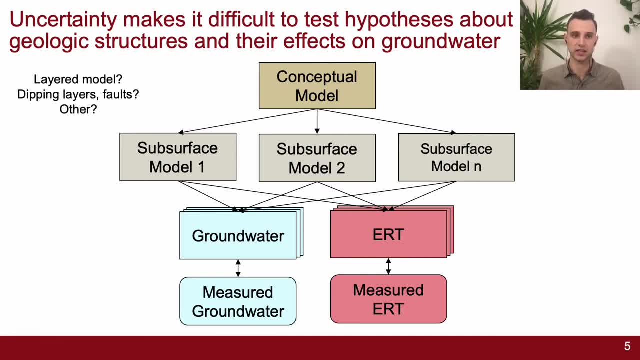 in. what kind of conceptual model do we use in the first place? so do we use this layered model? do we include geologic structures? how are we parameterizing our subsurface? and then, even once we've chosen a subsurface model, we have to parameterize it with layer. 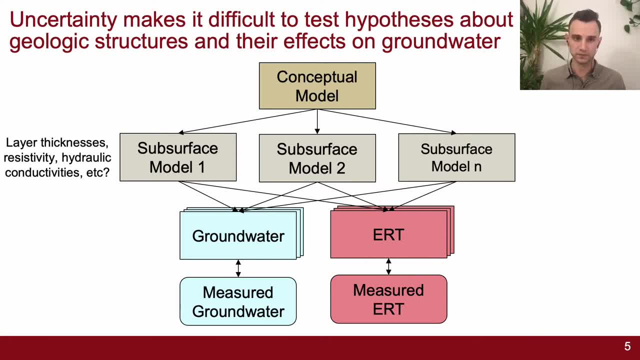 thicknesses, hydraulic properties etc. and those have uncertainties. but then when we go to actually ground water flow, we're going to have uncertainties on the forcings and the boundary conditions that we also have to account for. and then, to top it all off, we have error in our 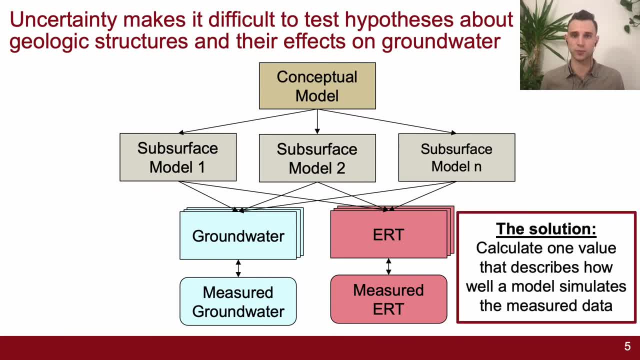 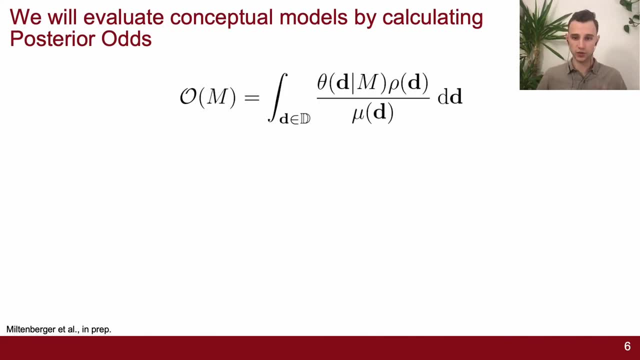 measurements that we have to account for as well. so the way we're going to approach this problem is to, for each conceptual model, we're going to calculate one value that describes how well that conceptual model is recreating our observed data, and so the way that we're going to calculate this- 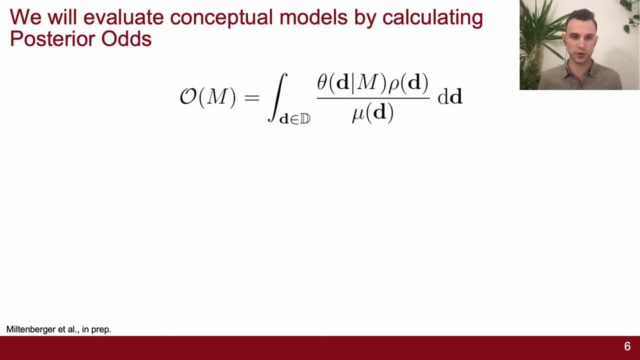 value is through the posterior odds, so we're going to calculate this value through the posterior odds. so the posterior odds is denoted by this here, where the o is the odds and then the m represents our conceptual subsurface model and the- the definition of the odds- is the posterior. 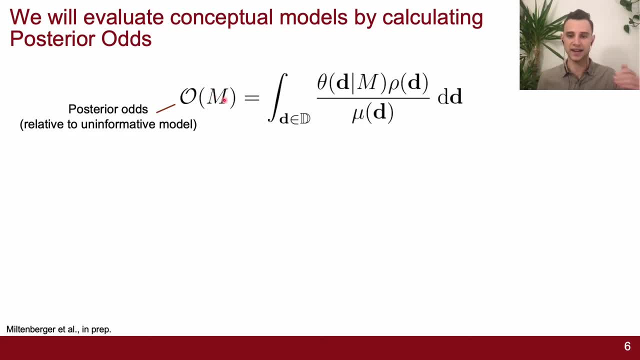 probability of that conceptual model divided by the posterior probability of an uninformative model. so this is, if we knew absolutely nothing about the subsurface. all we knew that we had was a, an er t measurement or a groundwater level measurement, but we knew nothing about what. 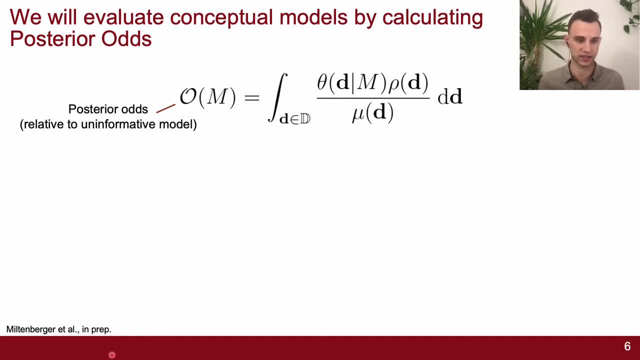 was controlling those measurements. that's what the uninformative model is telling us. so we're preparing a manuscript that describes some of this theory in more detail. but just to outline how we're going to do this calculation, we're going to take our modeled probability density of our data and then we're going to multiply that by the. 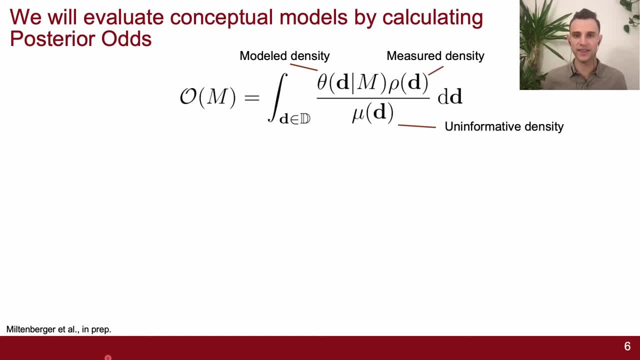 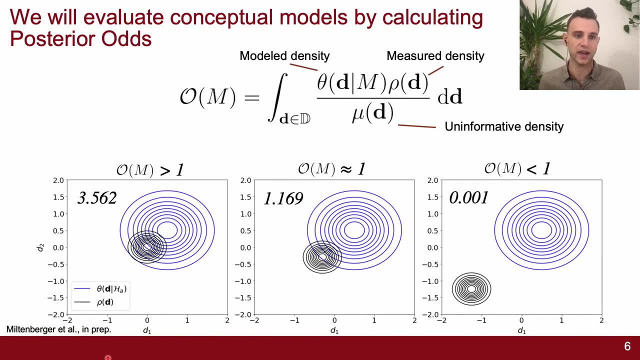 probability density of our measurements, divide that by an uninformative density, which is essentially Jeffrey's prior for those of you who have experience with Bayesian statistics, and then I wanted to show this example to illustrate intuitively what this posterior odds value is telling us. so here we have, our data in two. 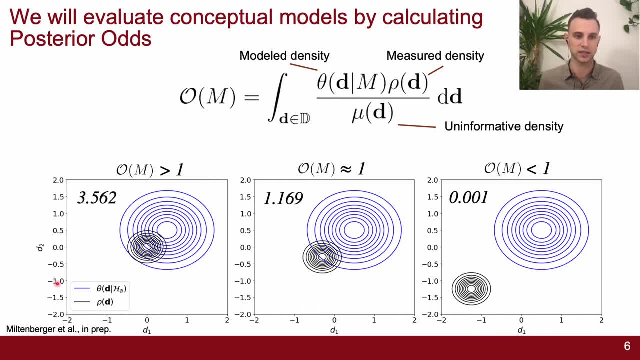 dimensions. so that's, it's plotted in in map view here. so we have data, one on our x-axis, our second data dimension on our y-axis, and our model density is shown in blue and our measured density is shown in black. so if we have overlap between our model and our data, then we'll get an. 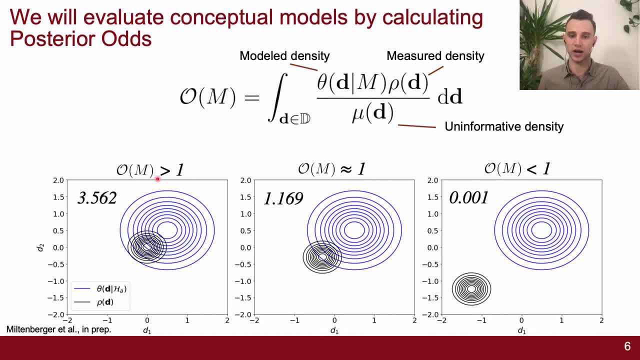 odds greater than one because the physical model is explaining the data better than an uninformative or random model. so in this case we end up with an odds of 3.562. greater than one model is doing a good job of representing the data. now, if we have some overlap, the model, the posterior odds. 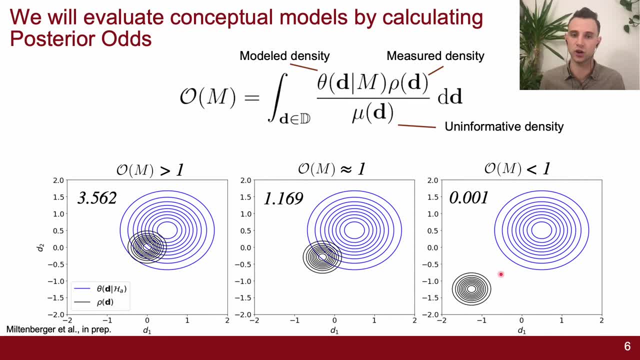 will be roughly equal to one, and then, if we have no overlap at all, then the posterior odds is less than one, which means a random model is doing better at explaining our data than a physical model is. so we need to reconsider our physical model. or something wrong with our intuition, so 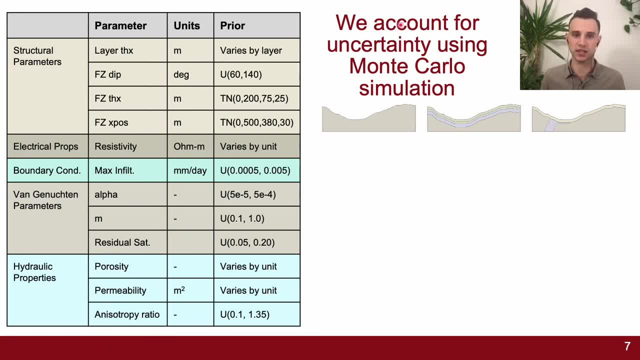 in practice. the way that we're going to do this calculation is we're going to use Monte Carlo simulation to simulate ERT and groundwater data, and that's what we're going to do here. so we're going to start off by doing a nice run on data to do aış. 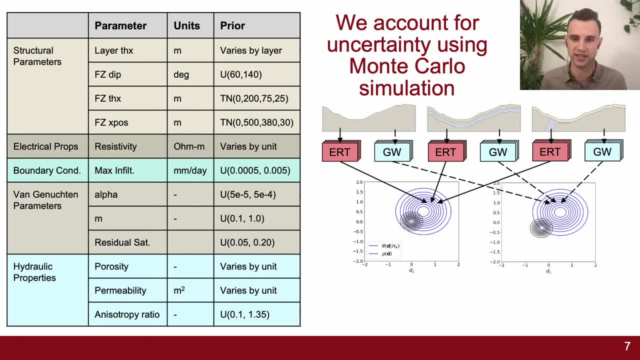 and so this table on the left just shows all the different parameters that go into it. we define uncertainties on all of these different parameters. there's 36 different parameters, but we've classified them into five categories here, depending on what kind of parameter they are. and so once we've done, our ERT measurements into a low dimensional space. then we'll do the same with our groundwater measurement and we'll go down to our görex, and now we're going to start to do our ground water measurement. so and so, once we have done this ensemble simulation and we have all of our realizations, we'll project our ERT. 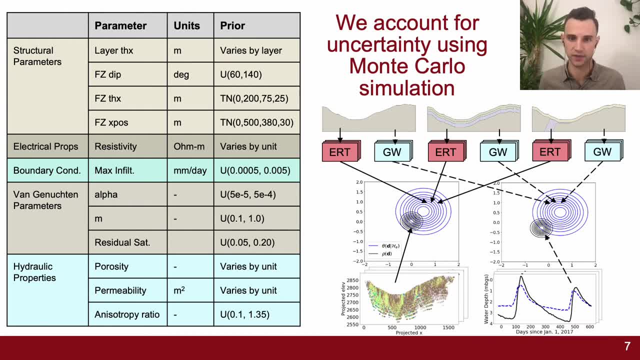 measurements into a low dimensional space, then we'll do the same with our groundwater measurement. that's what we're going to do here. so our structural measurement is going to be able to do as follows: we're going to do this and we'll bring in our measured data to compare and calculate that odds. 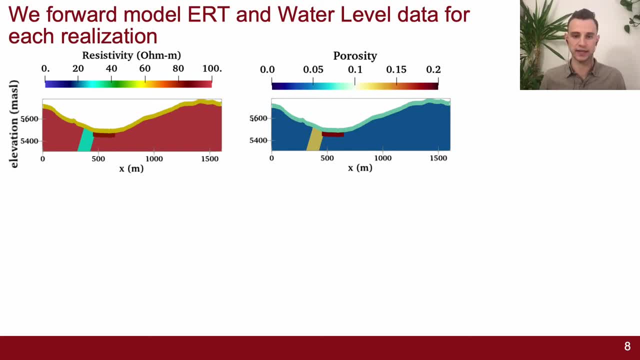 So here's an example of how we're going to do an individual simulation. We're going to populate a subsurface model with resistivity values as well as porosity, permeability and other hydraulic properties. We're going to use the resistivity to forward model electrical resistance measurements. 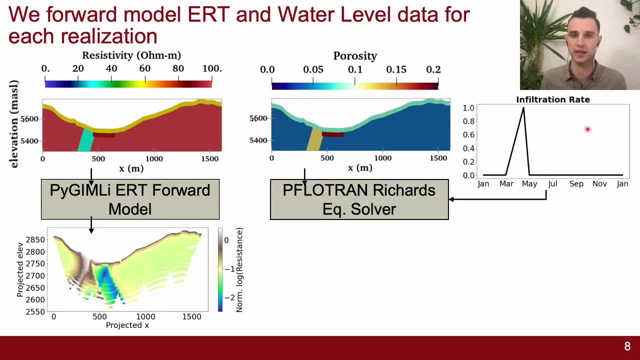 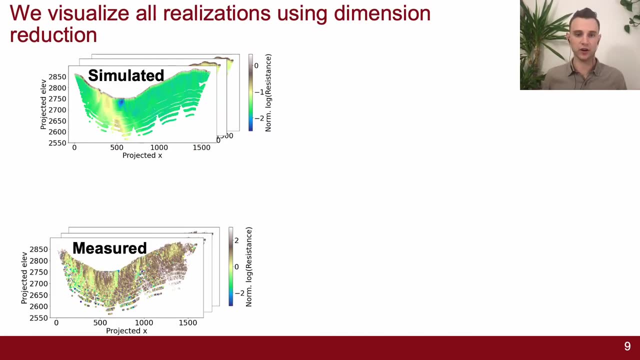 and then we're going to use our hydraulic properties, along with a boundary condition that simulates snowmelt infiltrating into the subsurface, and use a Richards equation, solver, to calculate water level data over the two-year period that we have observations. So when we have all of our Monte Carlo realizations created, 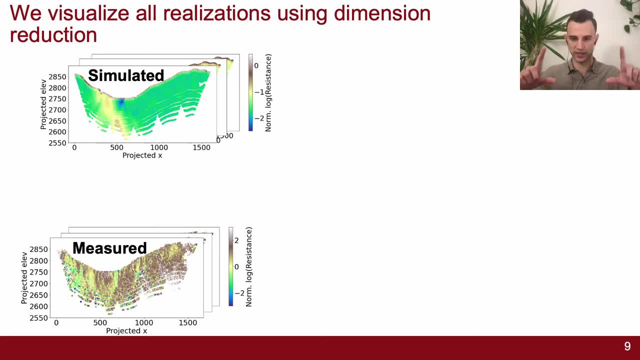 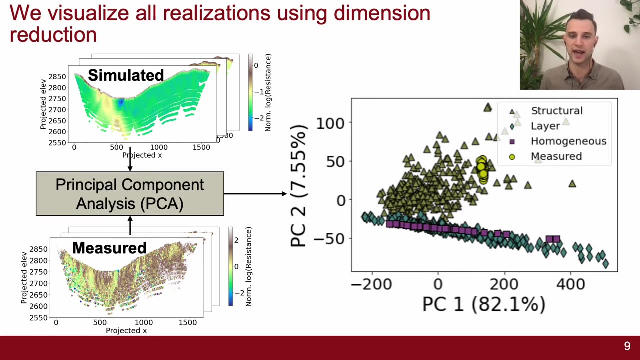 we're going to do dimension reduction so that we can visualize all of our realizations in one simple space. So what we're going to do is we're going to take our simulated data and draw realizations from our measured data using an error distribution and use principal component analysis to project them all into a low dimensional space. 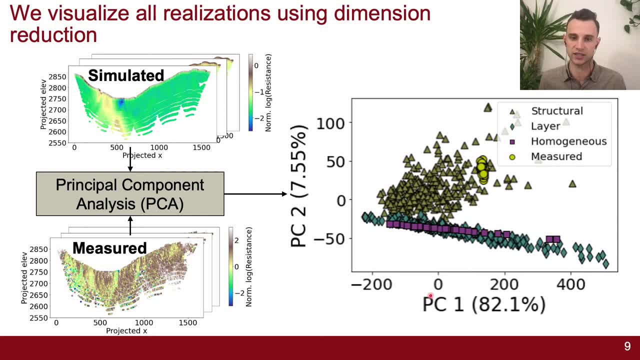 So in this case our first principal component is on the x-axis and our second principal component, score, is on the y-axis, and then our realizations are plotted as individual points in this reduced dimension space. So you can see, the measured data are in the circle. 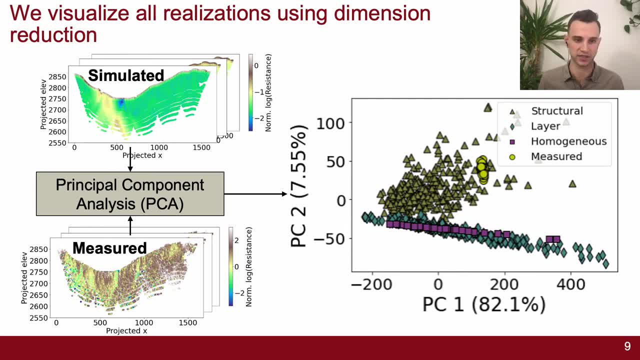 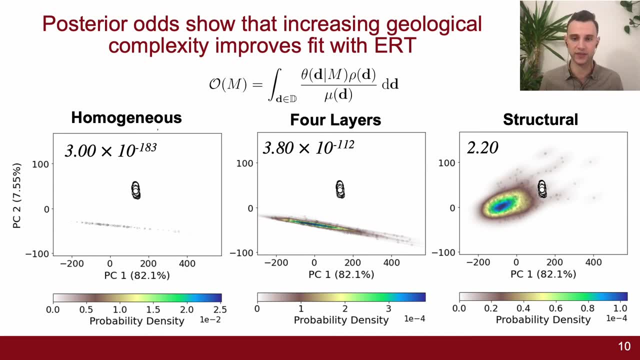 and then all of the simulated data are the rest of the symbols here, And so we'll go back to that equation for calculating the posterior odds, now that we've done everything, and we'll calculate the odds for each subsurface conceptual model. So that's what's shown with the numbers here in the top left corner. 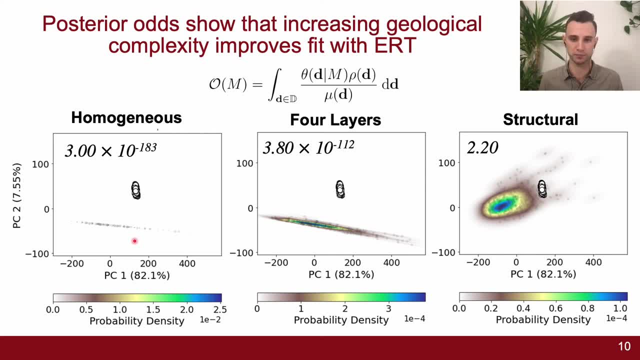 The plots themselves are just the same: principal components, score plots from the previous slide, except we've done kernel density estimation to estimate a probability density for each set of realizations, for each conceptual model. So you can see there's no overlap between the homogeneous model. 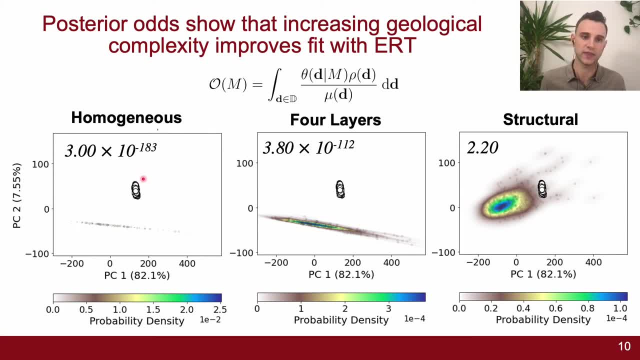 which is shown by these really faint circles and the measurements, which are the white larger circles, and so that gives us an odds basically zero, And it's a similar story for the layered model. it's not explaining our ERT data very well at all. 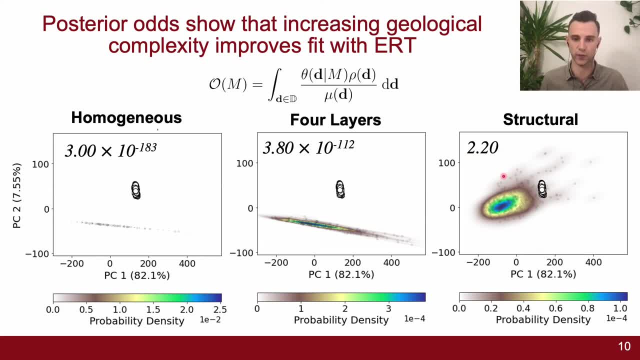 And it's not until we add the geological structure and that we're getting an odds that's greater than one, which means that our Physical model model is better than a random model, and that tells us that there's something to adding in this geological structure. there's something real about it because it's explaining our data pretty. 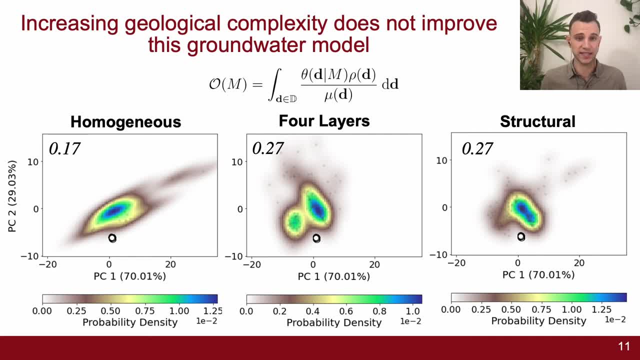 well. so, however, when we do the same thing with our groundwater level data, we get a different story. so the homogeneous model: we have an odds less than one, which tells us that our homogeneous model is not simulating our groundwater data very well. so we add in layers and we get a little bit. 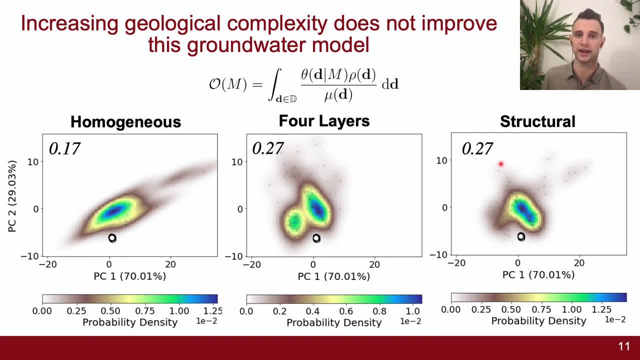 better, but adding in the structure doesn't improve over the layers at all. so what this is saying is that something about the these, the way we're setting up our groundwater model, isn't helping us simulate the observed water level data. so I want to show a couple of examples that show what's. 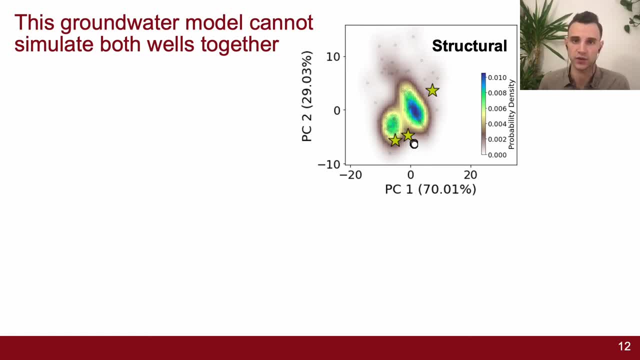 going wrong with the groundwater model here. so this is the same principal component score plot with the probability density overlaid from the previous slide for the structural model, and the stars here just show a couple of different realizations that I'm going to show next. so in this example we have the simulated water levels. 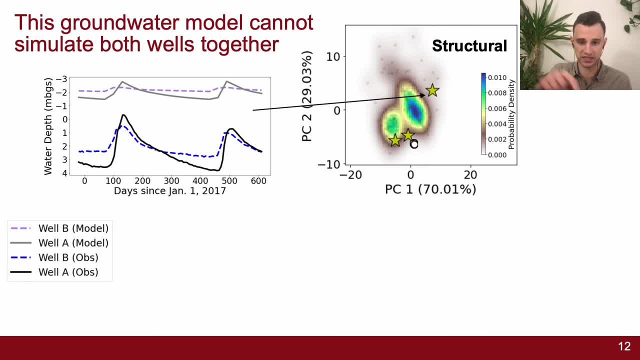 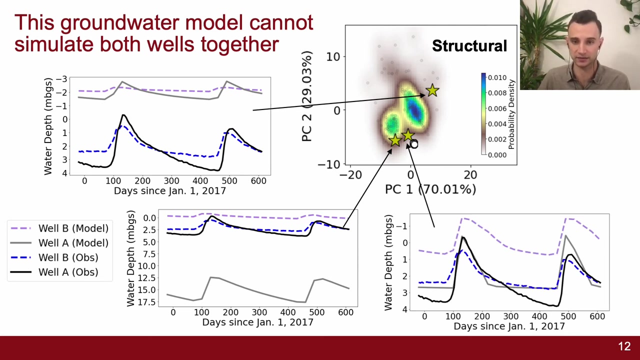 for well as a and B, following the same seasonal trend that we observe in the measurements, but it's offset by several meters. and then in this example, we have well B being simulated by the model pretty well, but well A is totally off. and then in this example, we have well A being simulated correctly, but well B is totally. 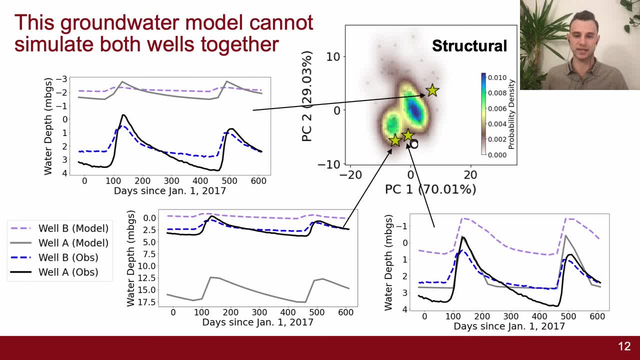 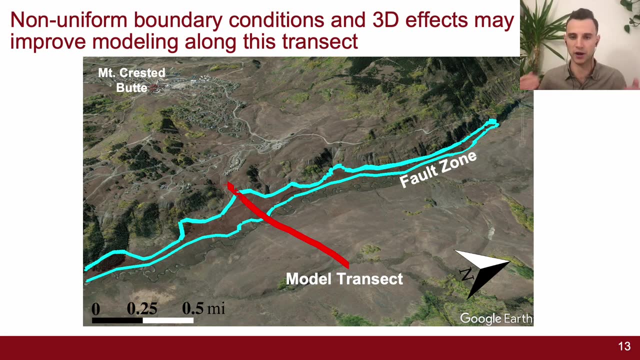 off, so we're unable to get both of the wells at the same time simulated. so there's something wrong with the way that our groundwater model is working, and so there's a few reasons why this could be happening, and the first is just the way that we're doing our 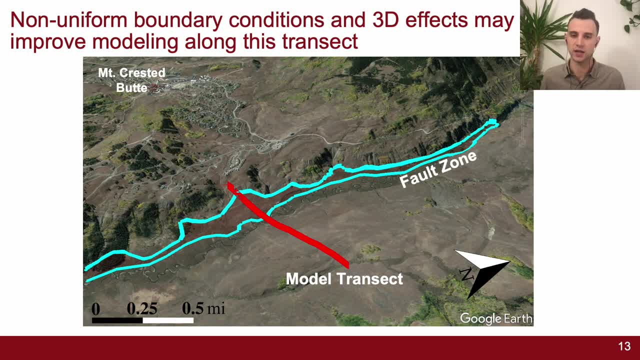 boundary conditions. we're using a spatially uniform infiltration rate, but in reality we know there's spatial variability that we just haven't modeled yet. so that's one of them, but there's other reasons, which is just due to the way that we're setting up the groundwater model. 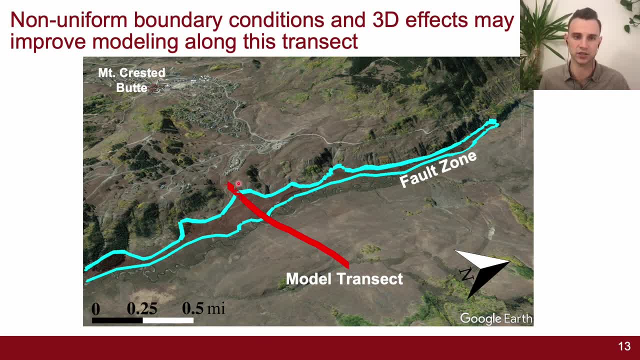 in the first place and that's what this slide is showing here. so our model transect is in red and then we stop the model at this, you know, somewhat arbitrary point. so we've completely excluded any effects from, you know, snow melt or or other things happening up. 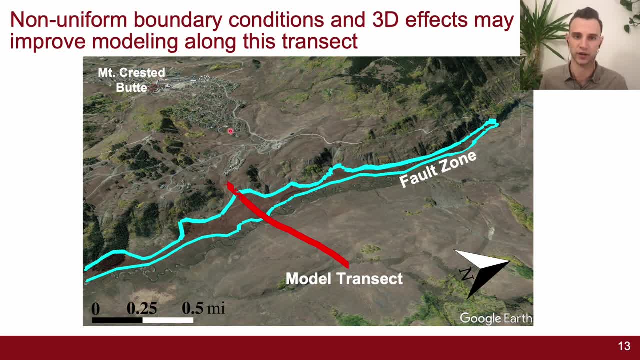 here in upslope from our model near the town of Mount Crested Butte or the surrounding mountains. and then we've also completely ignored this fault zone which we know from drilling is really hydraulically conductive, so there's even small hydraulic heads could result in a fairly 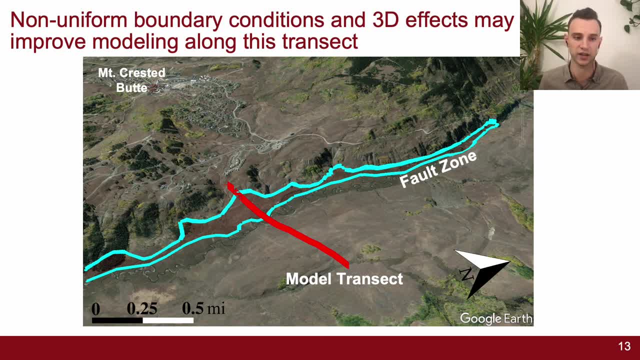 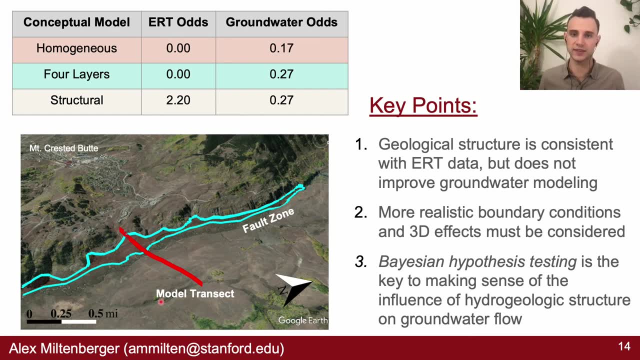 significant flow perpendicular to our model that we're never going to capture just using 2D. so that's one of the reasons why we're doing this, and the other reason why we're doing this is because we want to make sure that we're doing everything up really fast. what we've shown is: 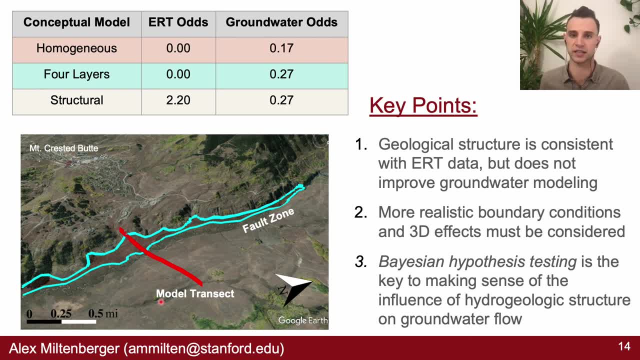 that in this case, our geological structure is real, it's, it's there, but including it is not improving our groundwater model along this particular transect. so we have to consider things like better boundary conditions and 3D effects. but I think really the key point from 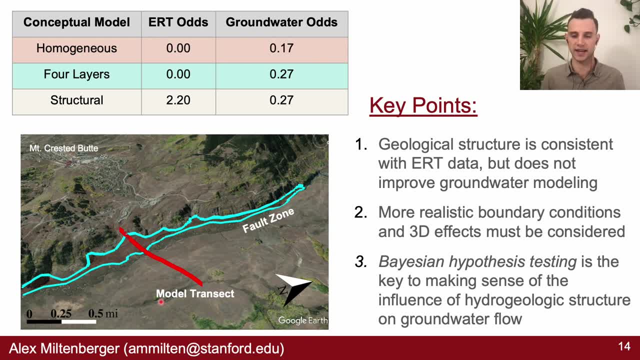 this work so far is that the Bayesian hypothesis testing- testing the act of going through and measuring geological structure- is impacting our groundwater modeling strategy. so I'll leave it on this slide and feel free to reach out to me. my email is in the bottom left corner. here I'll 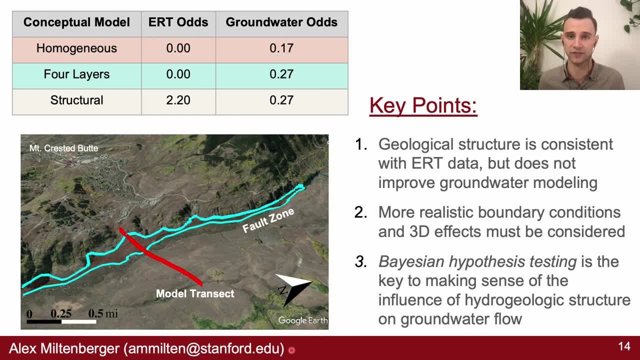 also be at AGU in person, and I'm more than happy to talk if anyone has any questions about this particular work or has any similar interests or anything as well. so thank you very much and I hope to see a lot of you in person in New Orleans next week.